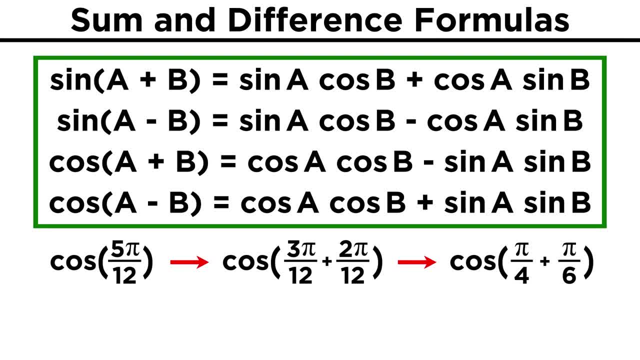 two twelfths pi, which reduce to quarter pi and a sixth pi. these are indeed angles for which we know precise sine and cosine values. So let's take this formula here and use quarter pi for alpha and a sixth pi for beta. 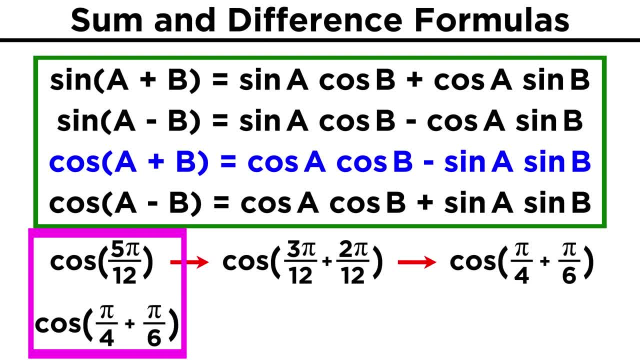 The cosine of the sum of these angles, which is the five twelfths pi we want to know about, will be equal to the cosine of quarter pi. This is not part of the unit circle, but if we split it up into three twelfths pi and 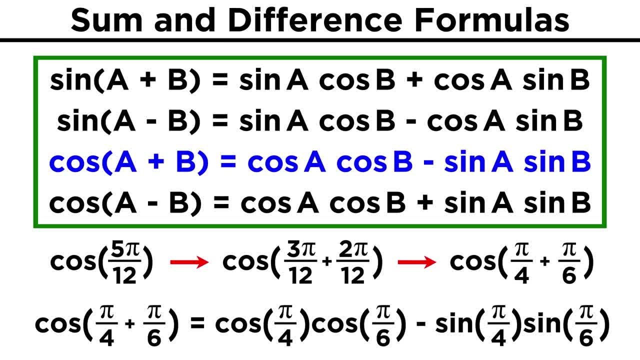 two twelfths pi times the cosine of a sixth pi, minus the sine of quarter pi times the sine of a sixth pi. Ideally, we have these values memorized from the unit circle. If not, go back and check out my tutorial on this subject. 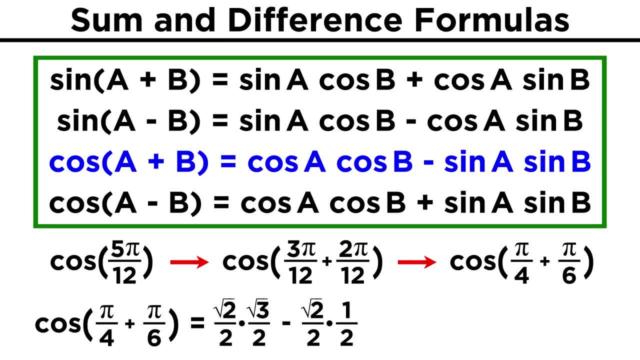 Otherwise we can just plug them in. They will be root two over two times root three over two, minus root two over two times one half. After multiplying, that's root six over four minus one half. That's four minus root two over four, which combine to give root six minus root two over. 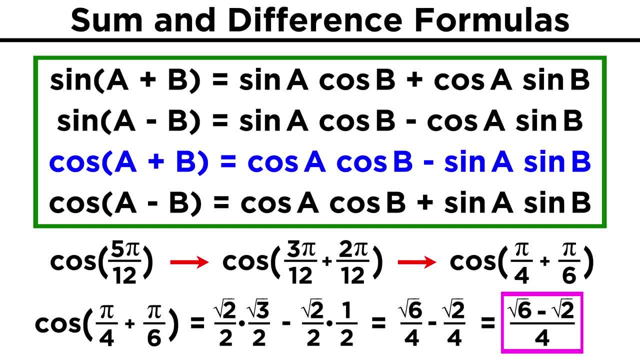 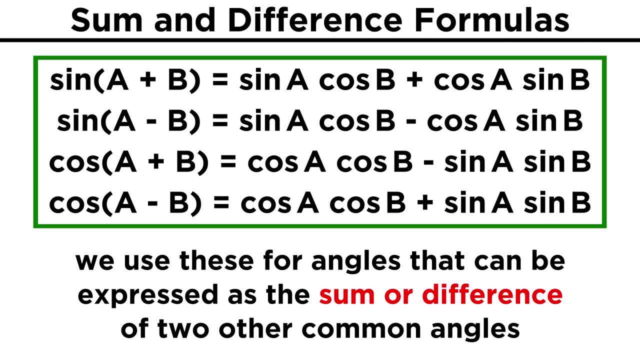 four. I know this isn't pretty, but it is an exact value which can be more valuable than approximating with a calculator. The other three formulas work exactly the same way. we just take the angle of interest and express it as the sum or difference of two angles that are more convenient to evaluate. 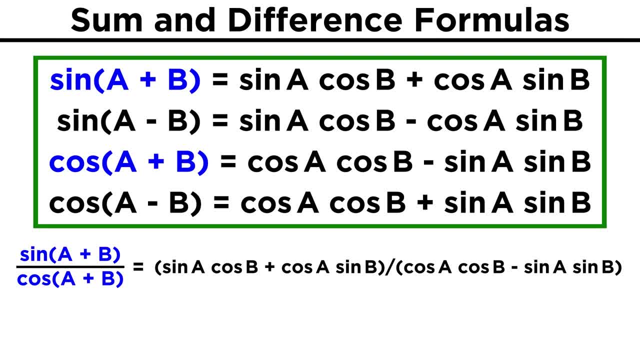 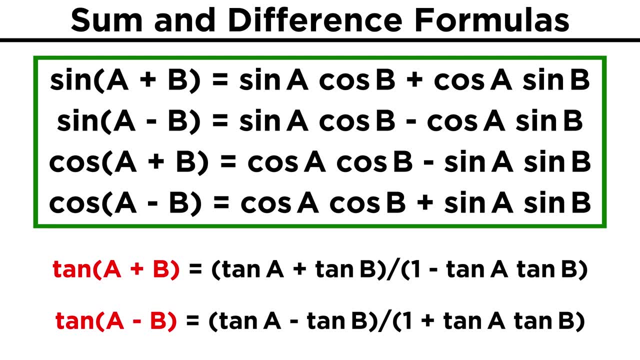 Also, if we place the sine of a sum over cosine of a sum, as well as the sine of a difference over the cosine of a difference, and do a little manipulation, we can get the sum and difference formulas for tangents as well, which look like this: 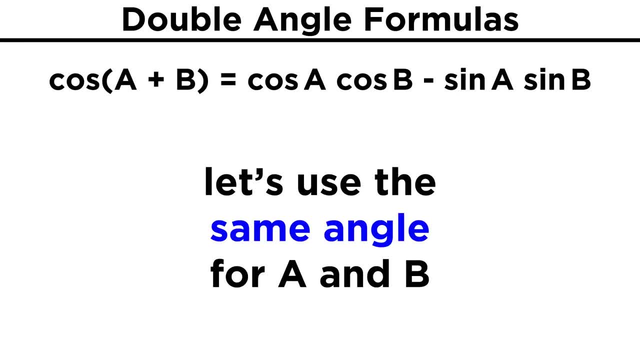 Next, let's look at double angle formulas. These can be derived if we use the sum formulas and plug in the same angle for alpha and beta. These can be derived if we use the sum formulas and plug in the same angle for alpha and beta. 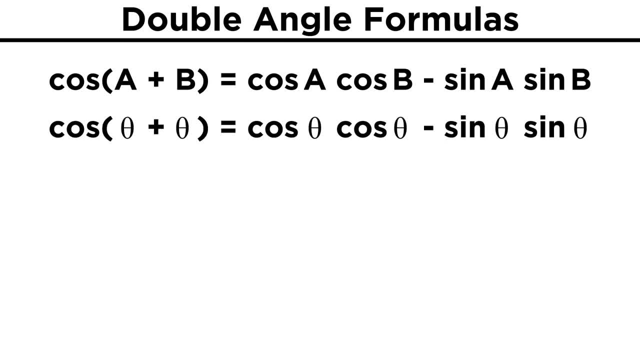 Looking at cosine first, let's put a theta in the place of all the alphas and betas. Alpha plus beta becomes two theta and that will equal cosine squared theta minus sine squared theta. so that's the double angle formula for cosine. 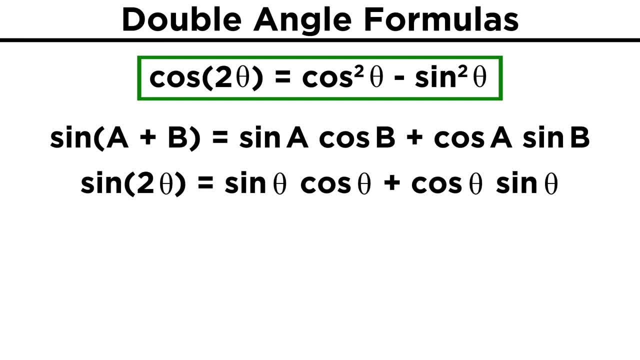 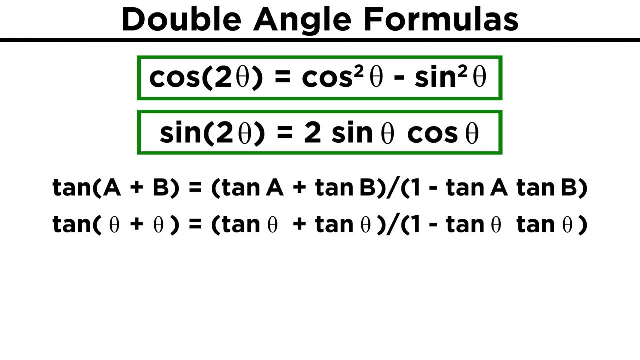 If we do the same for sine, we get the sine of two theta equals sine theta, cosine theta, plus sine theta, cosine theta, so that's two sine theta, cosine theta. Lastly, for tangent, we get tangent two theta equals two tangent theta over one minus tangent. 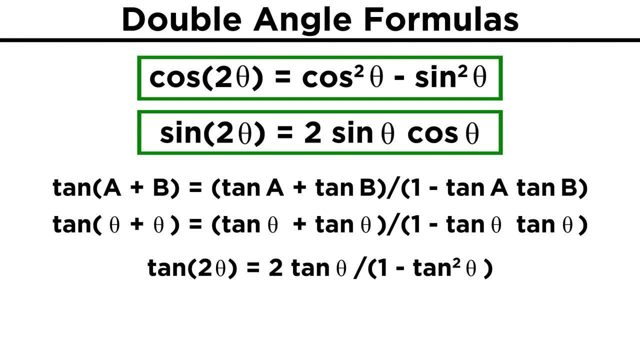 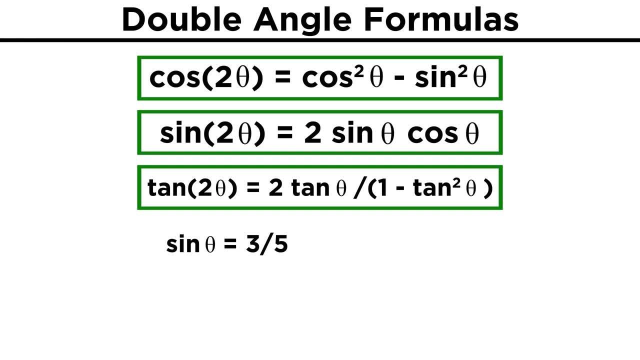 squared theta. These are easy to use. Let's say, we know that the sine of an angle lying in quadrant one is three over five. What will be the sine of twice that angle? Well, if we know two sides of the triangle, we know the third. it must be four. 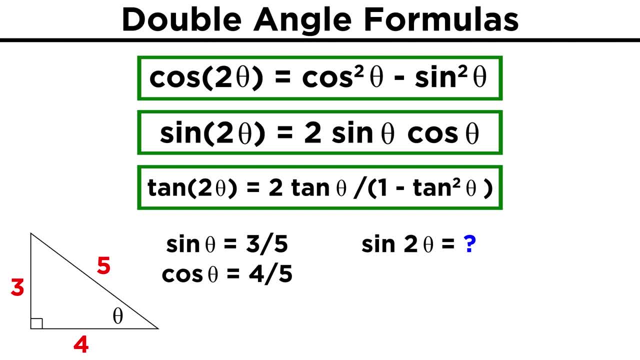 So cosine theta must be four over five. We just plug these into the formula and we get two times three, fifths times four, fifths, which is twenty-four twenty-fifths. We should also note that there are multiple forms of the double angle formula for cosine, because 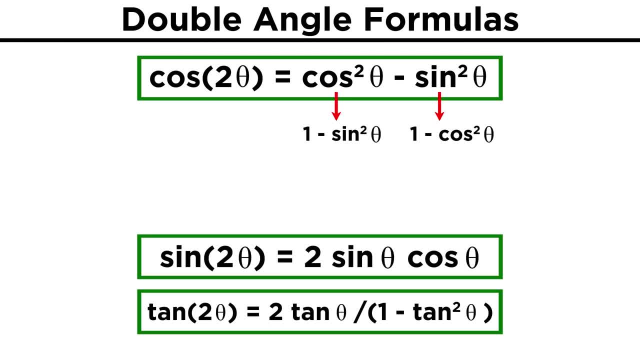 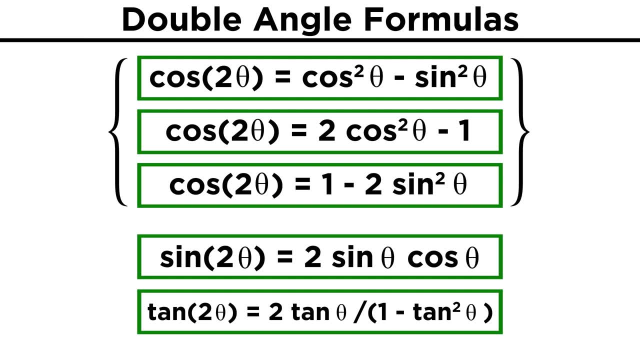 cosine squared can be expressed as one minus sine squared and sine squared can be expressed as one minus cosine squared. So here are the three forms for that, one being the original and two more given the two transformations we just mentioned. Now we can actually take these other two forms of the double angle formula for cosine and. 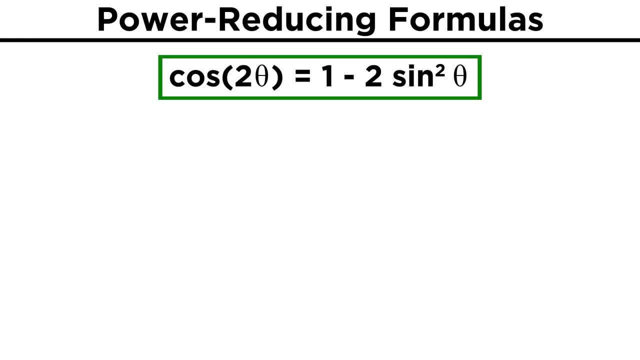 do something interesting, Starting with cosine two. theta equals one minus two sine squared theta. we get cosine two: theta equals one minus two sine squared theta. Let's solve for sine squared theta. We bring this sine term over here, bring the cosine term over there, divide by two and 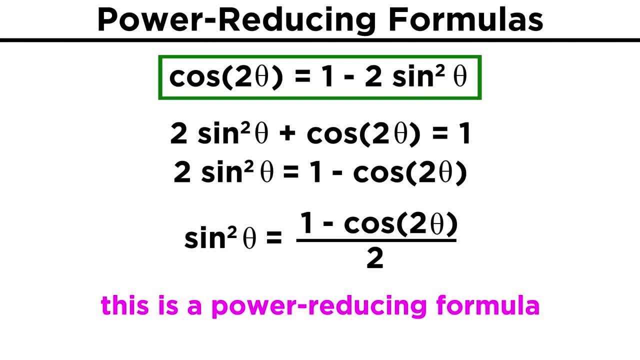 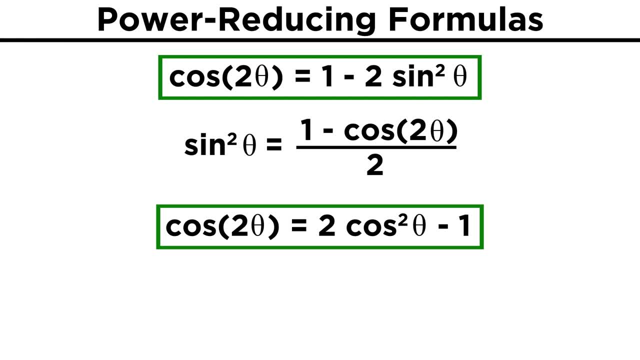 we have something called a power reducing formula. It allows us to express sine squared theta in terms of cosine theta. Let's do the same thing for this other form. bring the one to the other side, divide by two and we have cosine two theta. 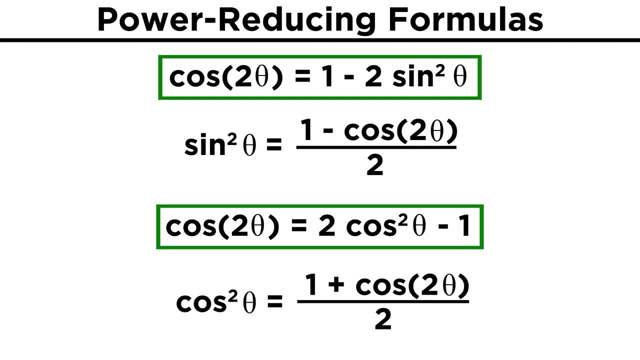 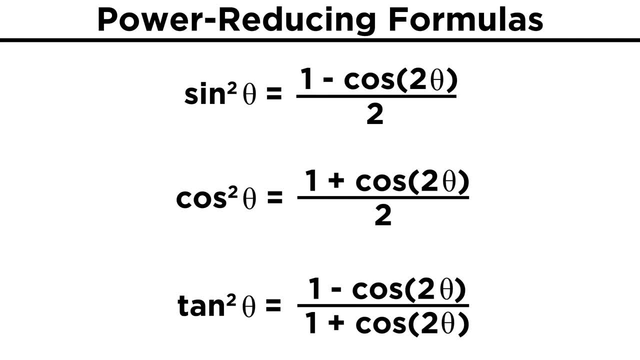 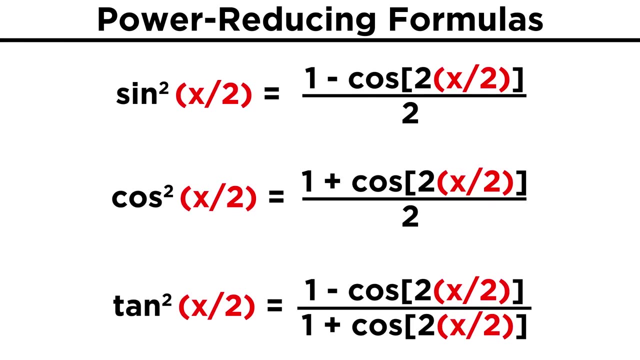 We have cosine squared theta in terms of cosine theta. Combining them gives us one for tangent squared theta. These expressions are useful in their own right, especially in calculus, but if we continue along with them, we can do another interesting thing. Let's say that for each of these we plug in x over two instead of theta. 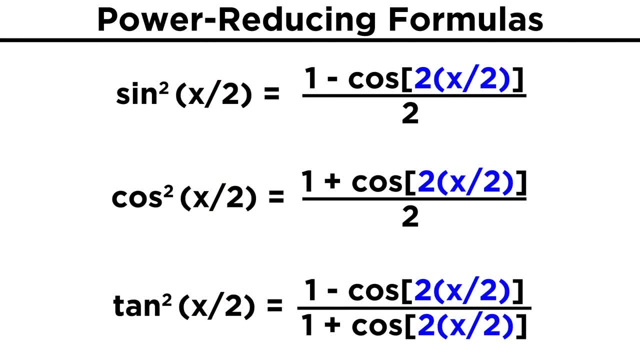 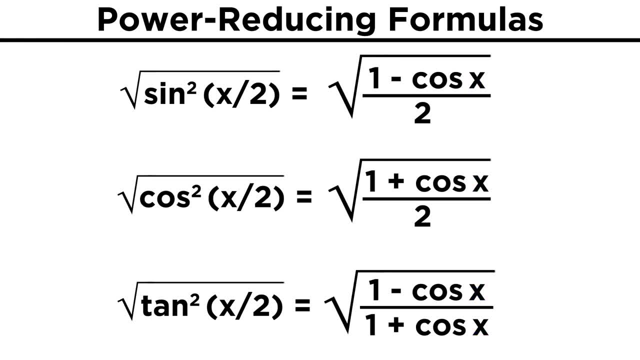 They will look more or less the same, except that all of the cosine two theta terms are cosine x. Then we can take the square root of both sides, and on the left we just get sine cosine and tangent of x over two. 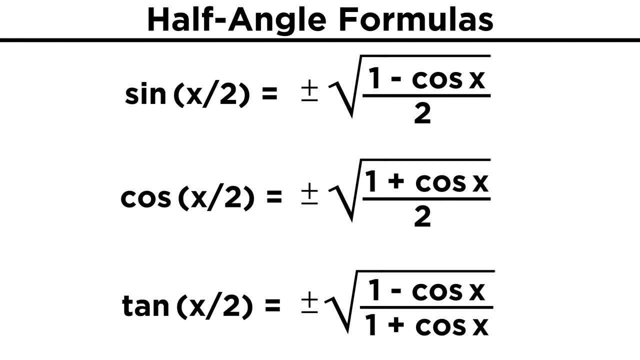 These are called half-angle formulas. They allow us to evaluate trig functions for smaller angles in terms of bigger ones with known values. and these plus or minus signs before the radical just mean that we have to look at the quadrant we are in to assign positive or negative. 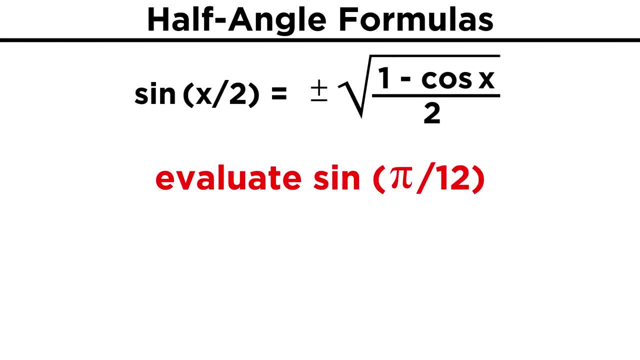 Let's do this, For example: what is the sine of one twelfth pi? Well, that's not on the unit circle, but one sixth pi is, which is twice this angle. So the sine of one twelfth pi is equal to the square root of one, minus the cosine of. 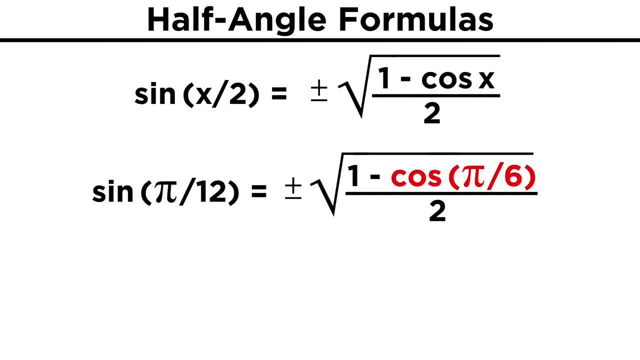 a sixth pi over two. The cosine of a sixth pi is root three over two, so we have one minus root, three over two over two. inside the radical Let's turn one into two over two, So that we can combine these to get two minus root three over two over two again, which. 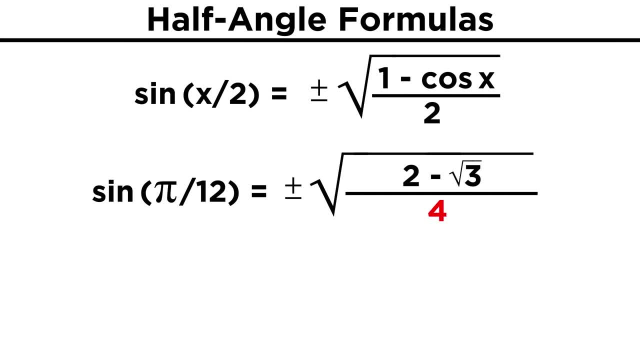 means two minus root, three over four. We can take the four out of the radical and we are left with a square root of two minus root, three all over two, which will be positive since we are in quadrant one. Not the prettiest thing to see a root within a root, but that's the exact answer. 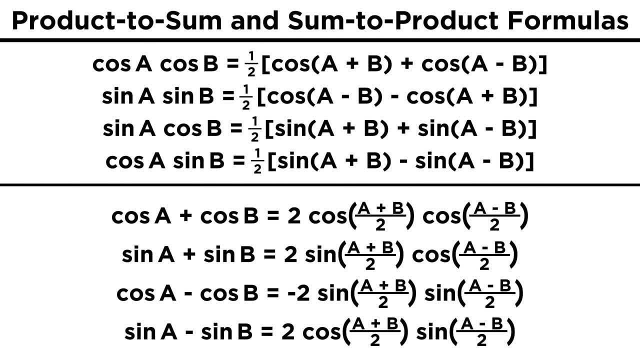 The last formulas we will look at are the product-to-sum and sum-to-product. These are exactly what they sound like. For product-to-sum formulas, each term on the left is the product of two trig functions involving two different angles. On the right, we have trig functions involving sums and differences.